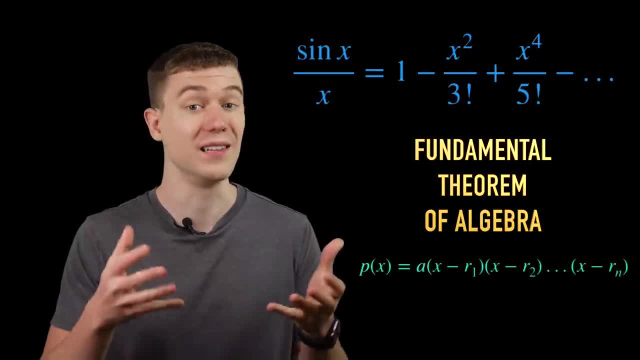 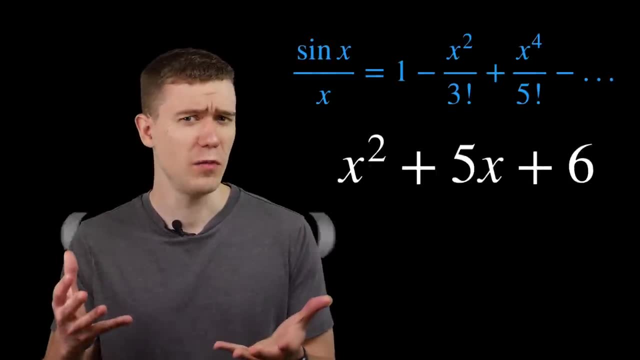 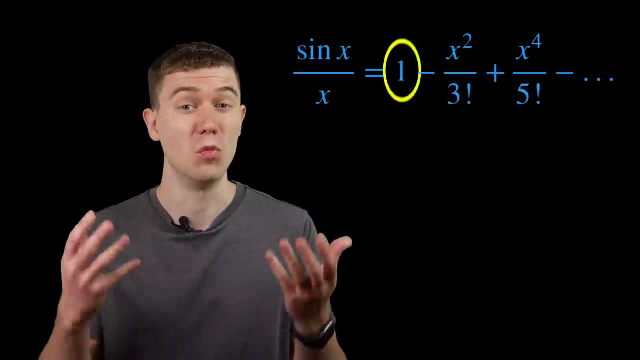 of algebra, We can factor polynomials into linear factors using the polynomial roots. Now think about how you factor basic polynomials. Typically, we think of two numbers which multiply to the constant term. The constant term of our polynomial is 1, and it's an infinite. 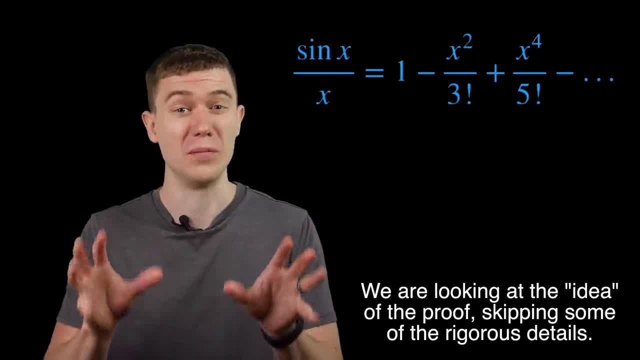 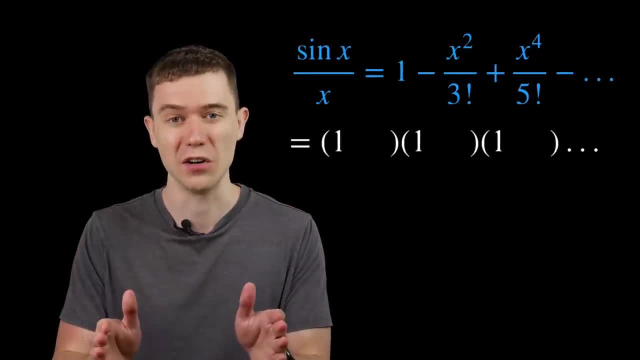 polynomial, so the numbers here all have to multiply to 1.. The only way that that's going to work- unless we want to use a bunch of fractions- is to make all the constant terms in the linear factors 1.. And we know when we plug in the roots, the zeros of the 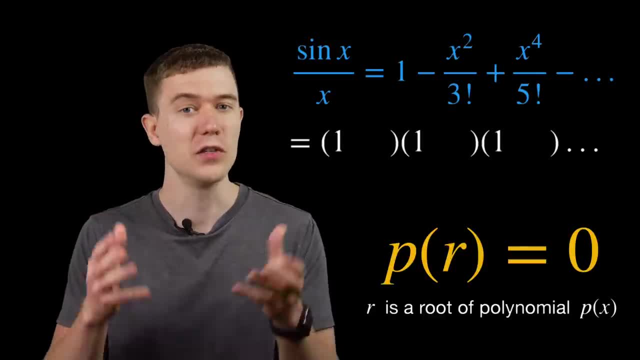 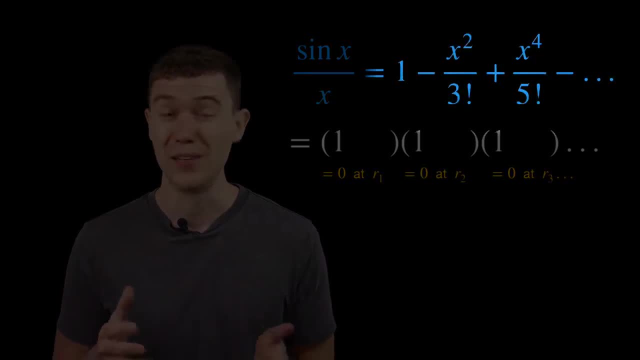 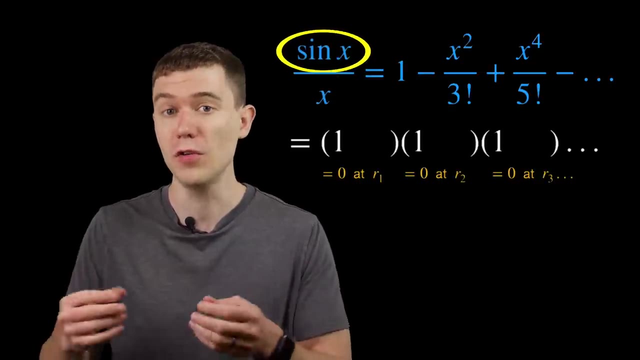 polynomial. for x it should be 0. So each factor should be 0 at one of the roots. What are the roots of this polynomial? Well, it's tough to see on the right hand side, but if we look at sine x over x, well that's 0 when the numerator is 0, and sine x is 0 at n times pi where n is an integer. 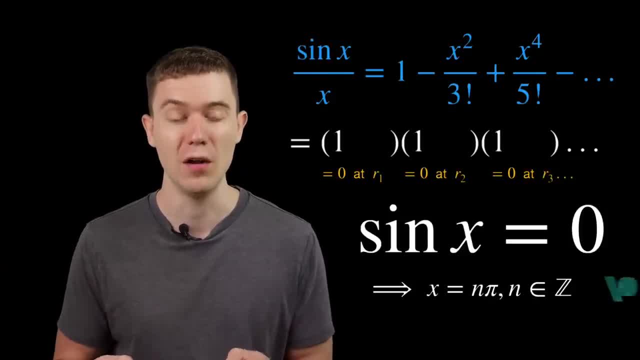 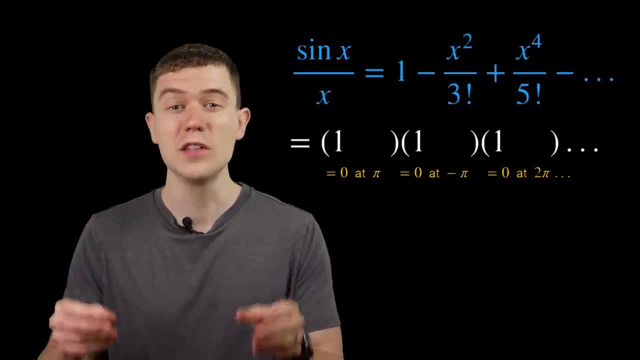 Well, we can't have 0 here, otherwise we'd be dividing by 0. But every non-zero integer is 0, so if we plug in the root of this polynomial we can get a root of the polynomial. So in other words, when we plug in plus or minus pi, plus or minus 2pi, plus or minus 3pi, and so on for x. 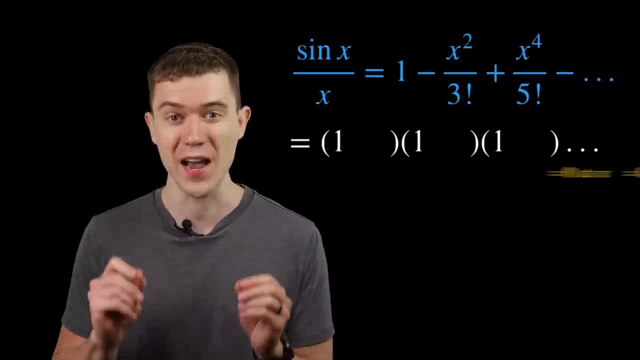 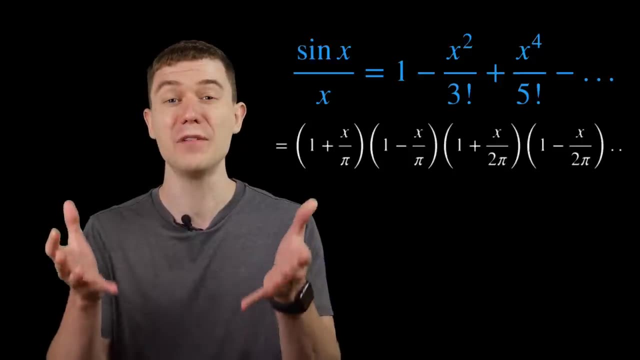 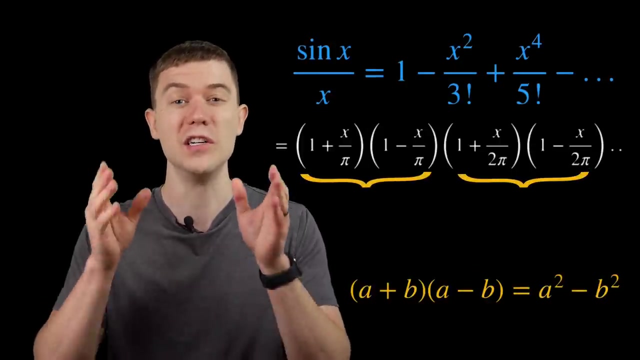 we have to get zeros at one of these factors. The way that we do that is make it 1 minus x over the root for all of the roots, And so we have the factorization here. If you're up to date on your factoring formulas, you may notice that this is factored into a bunch of difference of squares. 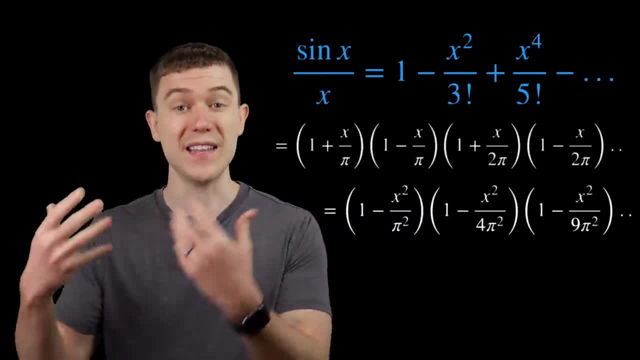 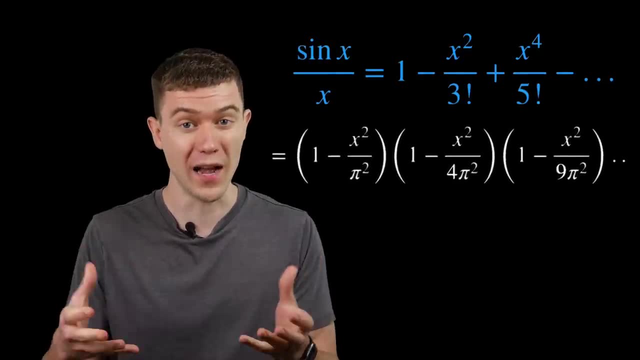 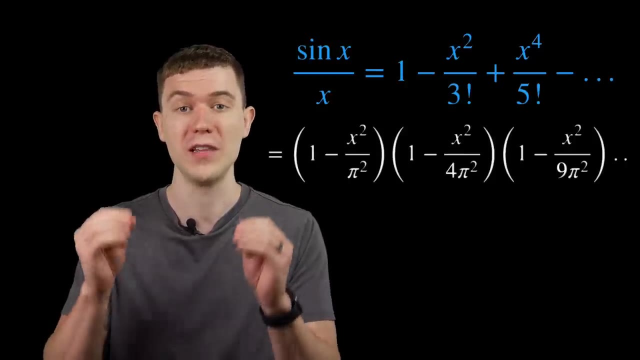 So each pair we can combine into 1 minus x squared over the root squared, and we have another factorization representation. If we were to multiply this all out and then collect all of the x squared terms, pull out the x squared term, the coefficient of the x squared term would be the minus 1 over pi. 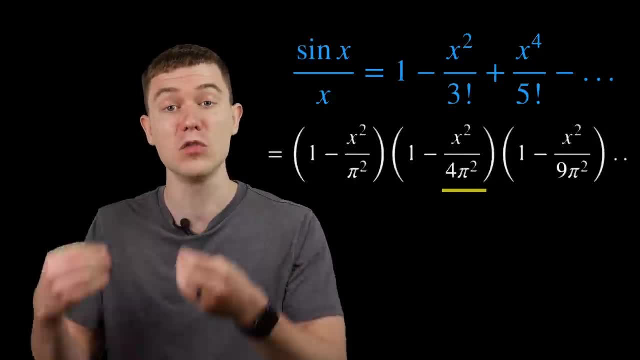 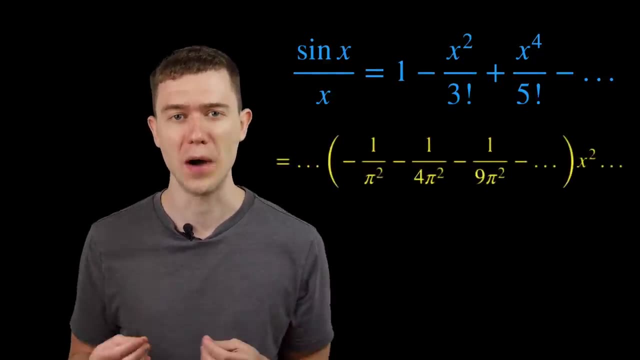 squared, minus 1 over 4 pi squared, minus 1 over 9 pi squared, and so on. So the coefficients all have a negative, they all have an over pi squared. factor out the minus 1 over pi squared and what we'll see is that coefficient is the sum we were actually.